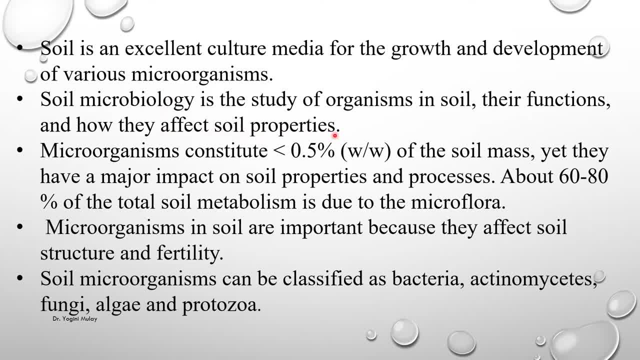 microorganisms affect the soil property. Microorganism constitutes less than 0.5% weight by weight of soil mass. Even if they are present in such a low number, such a low amount, they still have major impact on soil properties. About 60 to 80% of soil metabolism is due to the microorganism. 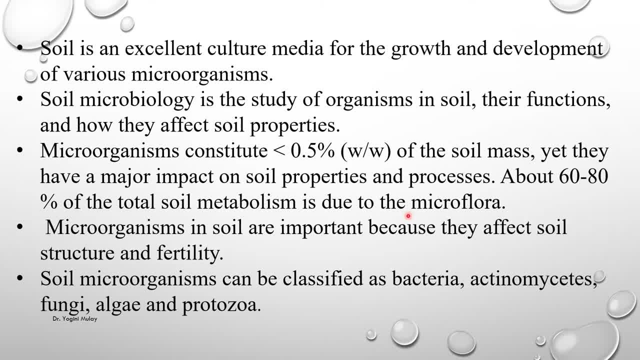 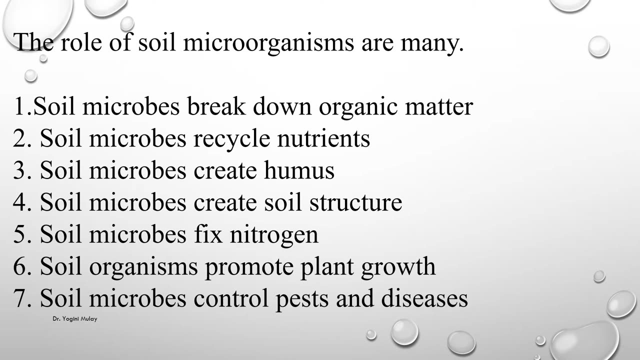 present In soil, these microorganisms. they determine the fertility of soil and these microorganisms are of five types: bacteria, actinomycetes, fungi, algae and protozoa. We will be dealing with each type of microorganism in detail. Before we go in detail about each type of microorganism. 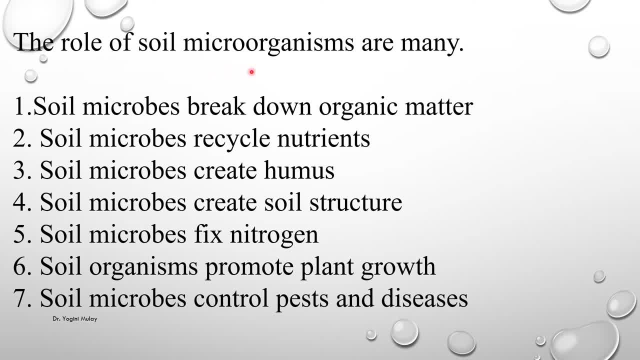 we must know the role of microorganisms. Let's start by discovering the role of these microorganisms in the soil: pta2, These soil microorganisms. they mainly involve in breakdown of organic matter. They contribute for the recycling of nutrients. They are responsible for creation of humus. They determine the soil. 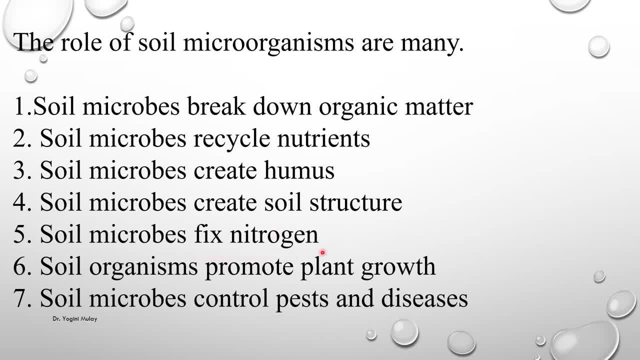 structures. They are responsible for fixation of nitrogen against dick. all of this is the root cause, node Niptonian, Niptonian Plant Organ. They promote the plant growth and they have an appreciable contribution in control of various plant diseases. Let's talk about the soil bacteria. 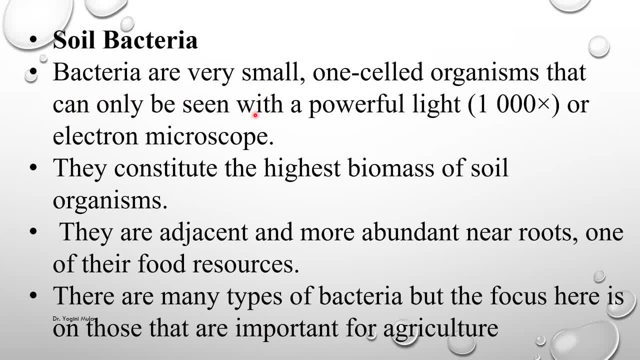 Bacteria are very small. They cannot be seen with our naked eyes. We need to take aid of powerful light or electron microscope. They constitute the highest biomass of soil organism. They are mainly present near the root of plants, because the excretion from the root is the main food resource for the bacteria. 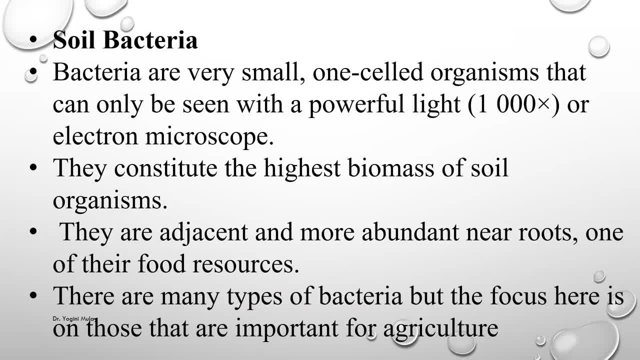 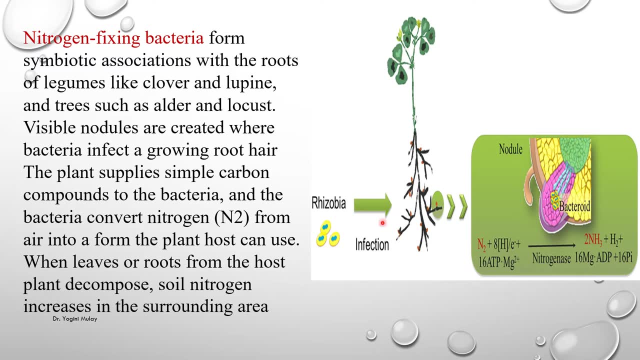 Actually there are many types of bacteria presence in the soil, But here we will focus only about the bacteria which are important From The point of view number one: nitrogen fixing bacteria. nitrogen fixing bacteria: they form symbiotic association with the roots. Here the visible nodules are formed and the these bacteria are presence in this nodule. 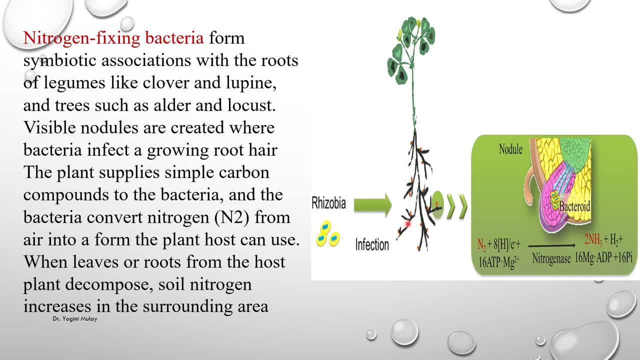 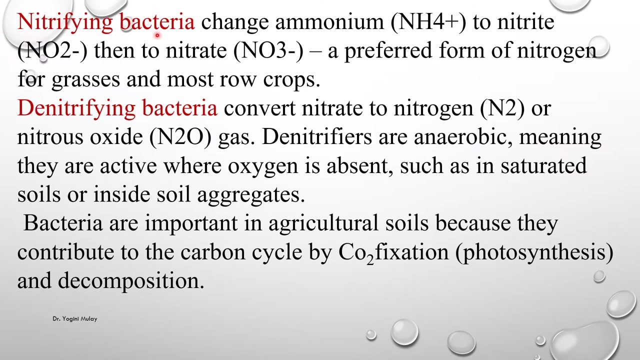 The plant supplies simple carbon compound to this bacteria. Where are these bacteria? they convert atmospheric nitrogen into ammonia, Into ammonium ion, and this is the form which can be utilized by the host. Second type of bacteria is nitrifying bacteria, As I mentioned in my previous slide. atmospheric nitrogen- 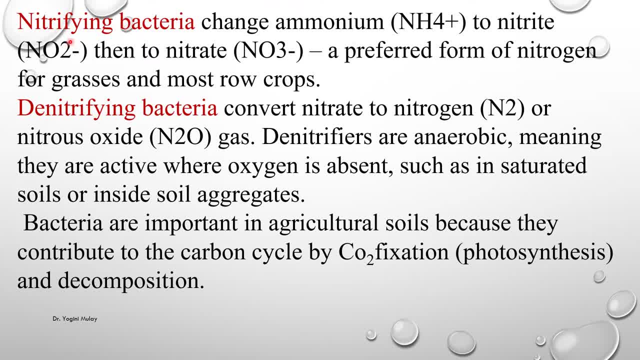 Get converted into ammonium. Now, these nitrifying bacteria, they convert ammonium into nitrate form, Which is all a preferred form of nitrogen for many of the crops. Next, love denitrifying bacteria. They are mainly on. it will ask and they convert this. 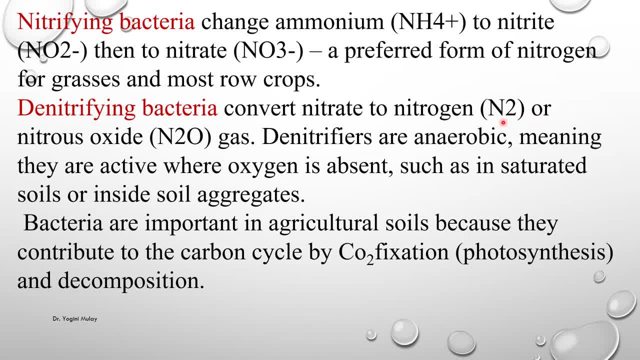 Nitrate into nitrogen. There are a lot of Motors and motorcycles. багnes, chiarin had a difference in this, the All eficiency criteria. they're mainly good as all populationillo a part vaccine. Thus the three types of bacteria, as we have seen: nitrogen fixing bacteria, nitrifying bacteria, denitrifying bacteria. they play important role in nitrogen cycle. 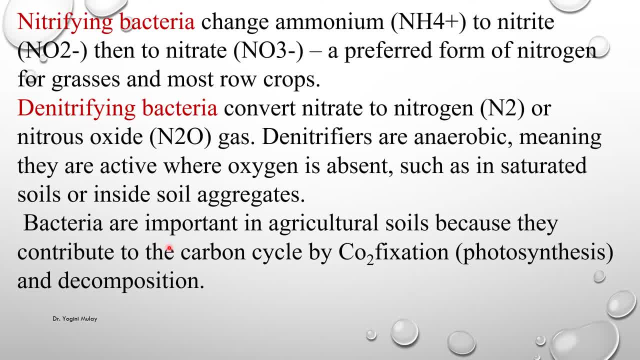 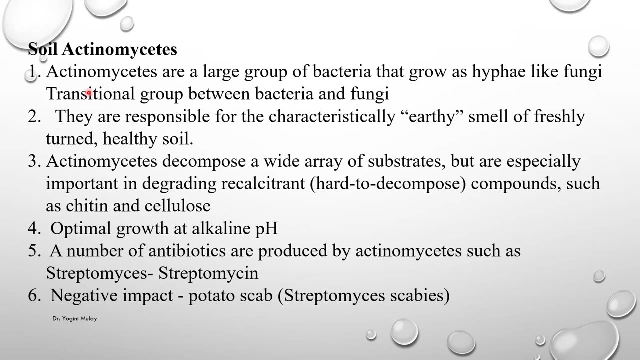 Bacteria plays important role in carbon cycle, also by the CO2 fixation that is, photosynthesis, as well as they contribute for the decomposition of many of the carbonaceous compound. Let's talk about the soil actinomyces First of all. what is actinomyces? 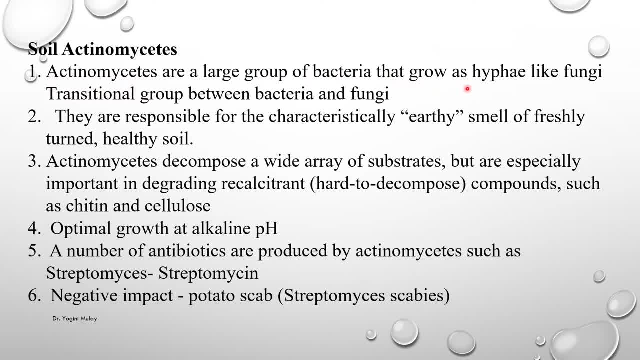 Actinomyces. it is a large group of bacteria that grow as a hyphae. like fungi, They show some properties which are similar to bacteria and, whereas some properties are similar to fungi, These actinomyces are mainly responsible for characteristically earthy smell of freshly turned, healthy soil. 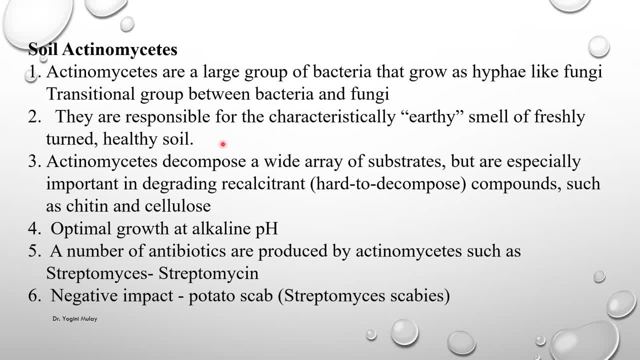 Means whenever the first rain falls. That time we get a very good smell from the soil and that is known as the earthy smell, and that is because of actinomyces presence in the soil. These actinomyces, they can decompose a wide variety of substrates. 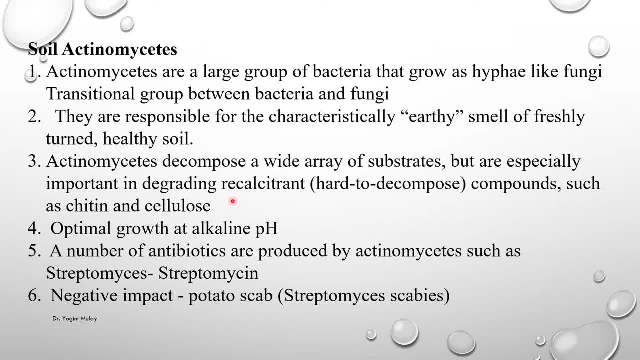 Especially they are important in degradation of recalcitrant means, the compounds which are really difficult, very hard to get decomposed, Such as chitin or cellulose, etc. Actinomyces: they can grow at alkaline pH, Means their optimum pH is alkaline. 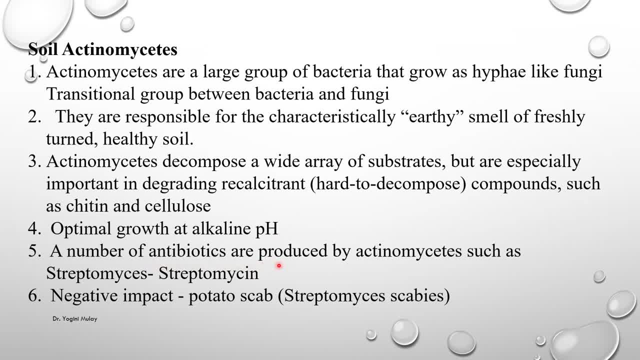 And they are capable of producing number of antibiotics Like. the well-known example is tryptomycin. It is antibiotic which is produced by tryptomyces. As we have seen that they mainly contribute by producing different types of antibiotics, they still have the 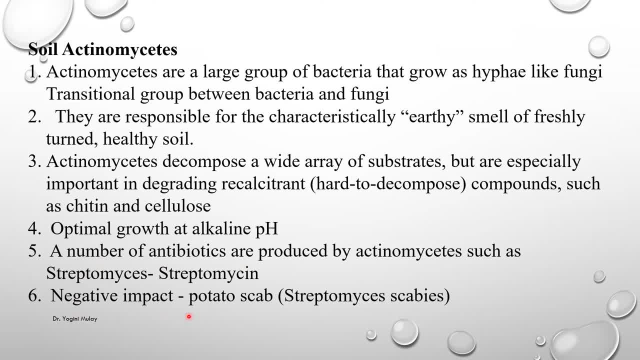 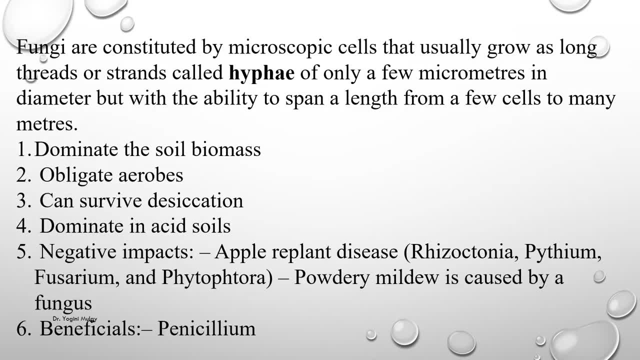 negative impact. They can cause the various diseases also. Example is potato scab. Next is fungi. Fungi are constituted by microscopic cells and they usually grow in the form of hyphae. They are dominant in the soil. biomass means they are present in large number. 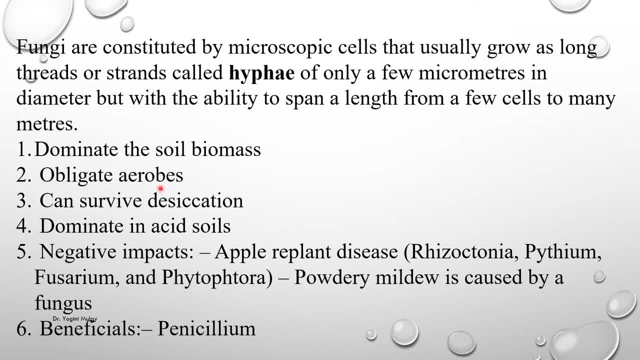 They are mainly obligate aerobes. They can survive in desiccation also. They mainly present in the acidic soil. They are responsible to cause various diseases to the plants. and from the beneficial point of view We look at the fungi. They are capable of producing the various types of antibiotic. 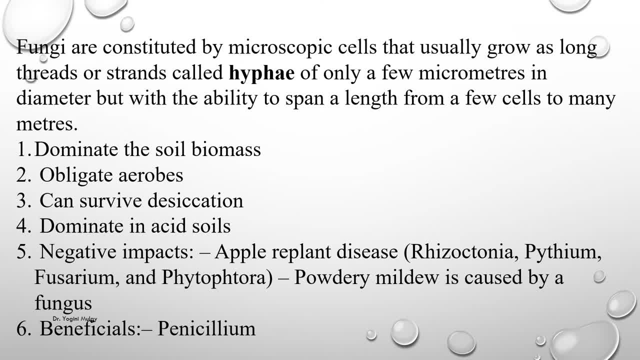 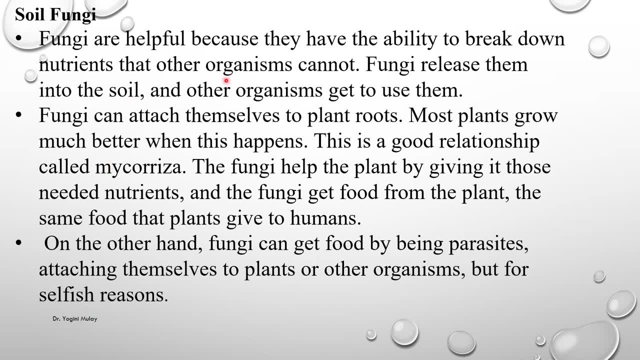 Example is penicillin antibiotic, which is produced by penicillium. These fungi are helpful because they have ability to break down the nutrients, and the fungi releases nutrients in the soil and the other organisms use it. They can attach themselves to the plant root. 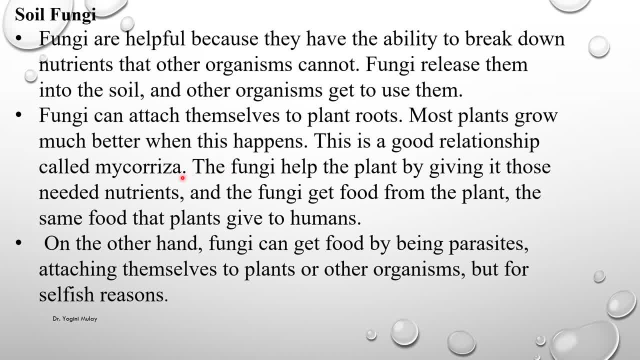 and this is the good relationship in between the fungi and plant root, and we call it as a mycorrhiza Here. the fungi help the plant by giving it to needed nutrients, whereas fungi get the food from the plant, The same food that plants gives to human. 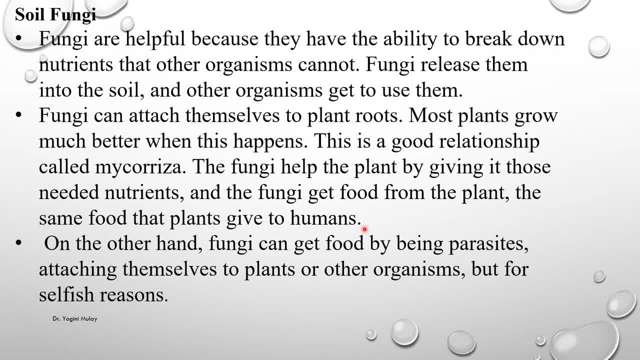 So this is the symbiotic relationship between fungi and plants. On the other hand, there are some examples of fungi which can get the food. by being a parasites means they attacked themselves to the plant or to other organisms, but this is for the selfish reason only. 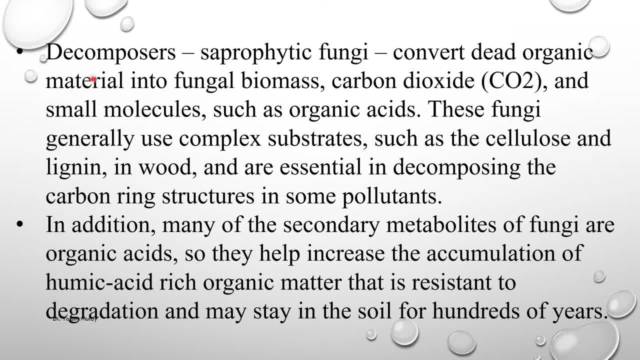 The major role played by the fungi is idealization. The major role played by the fungi is idealization. fungi are, they are decomposers, means we call it as a saprophytic fungi, as they convert dead organic material into the fungus biomass and into carbon dioxide, as well as some different types of. 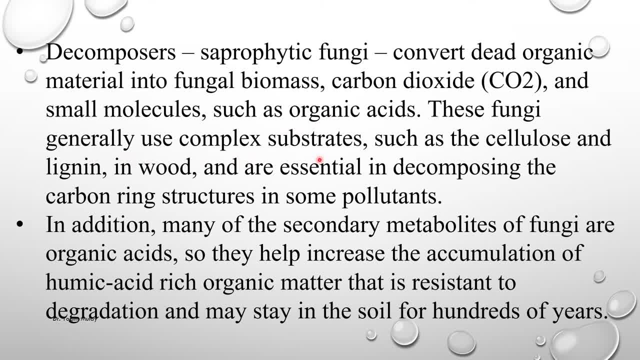 organic acids. These fungi generally use the complex substrates, such as cellulose lignin, which are present in the wood. In addition, they are capable of producing the secondary metabolites, like organic acids, and thus they help to increase the accumulation of humic acid rich organic matter. 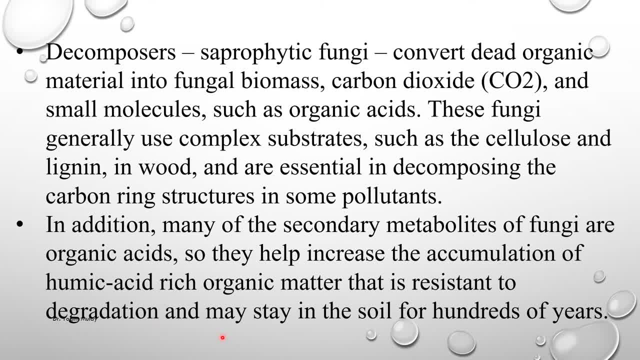 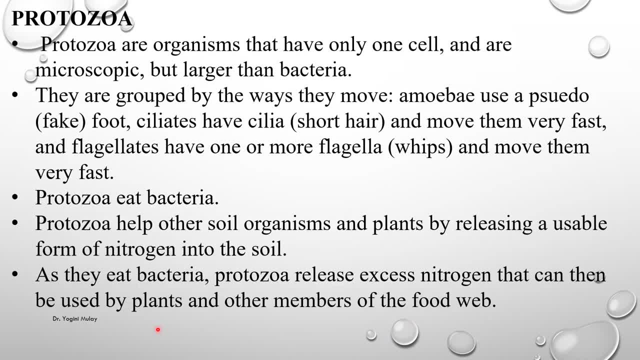 that is resistance to degradation, and they may stay in the soil for hundreds of years. Next is protozoa. Protozoa are organic organisms which are present in the form of one cell. They are microscopic, but they are larger than the bacteria. They are grouped by the ways they move, like amoeba. amoebae, they use the